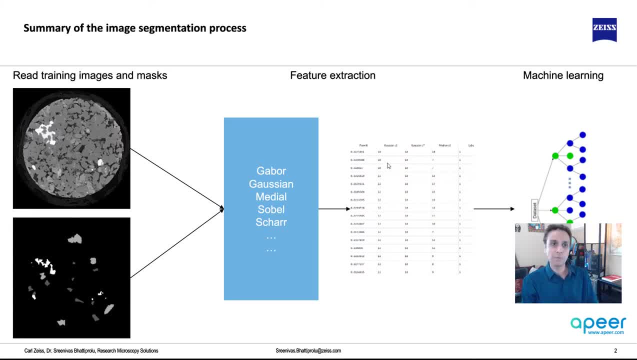 and then capture the responses as individual columns into a data frame and supply this data frame to a machine learning algorithm, in this case random forest- and in this process we dropped all the pixel values with a value of zero, because they represent areas that are not labeled because they do not contain any information. So that's what happened in the last tutorial. 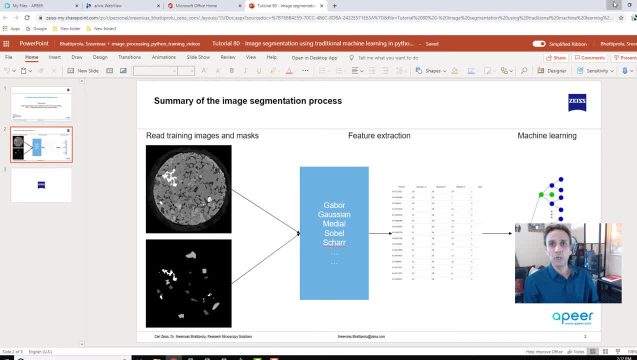 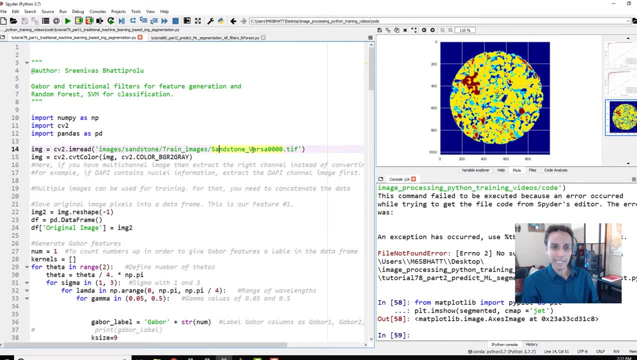 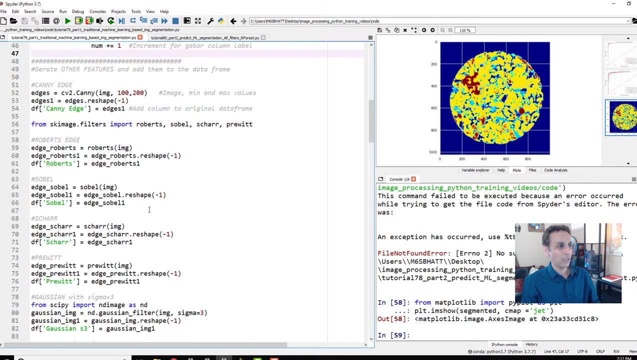 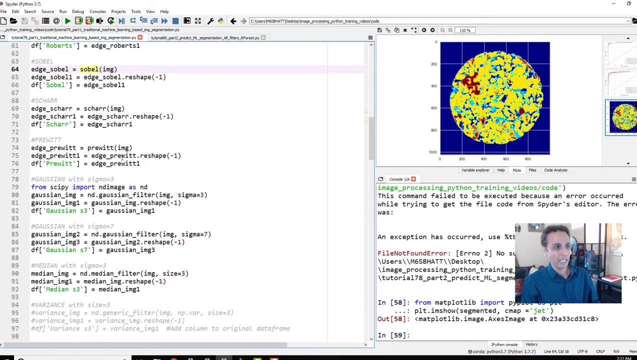 of course, in Python. So now let's jump into our Python IDE- and I still have this from my last tutorial- where, like I said, we loaded an image and we generated Gabor features- 32 of them- and to that we also added additional filtered responses from Kenny Edge, Robert Sobel, Shar Pruitt and Gaussian. 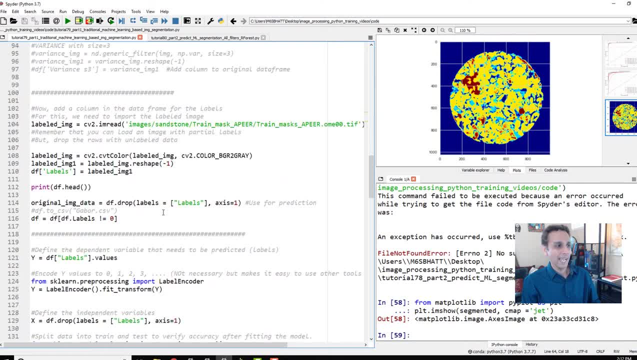 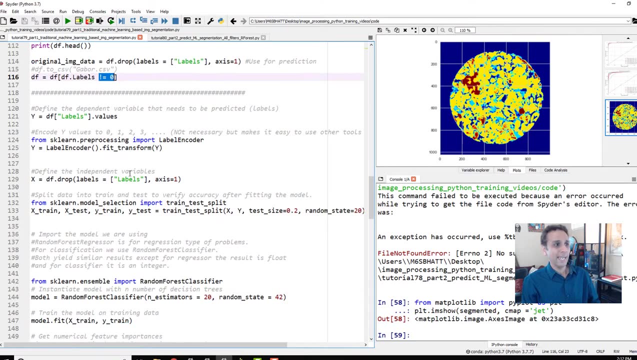 3, Sigma, Gaussian, 7, Sigma and median filtered. and then we also added a column of all the labels, so we know, you know what the ground truth is. and we dropped all the labels with a value of zero because they don't mean anything for this machine learning process. and then we also encoded the. 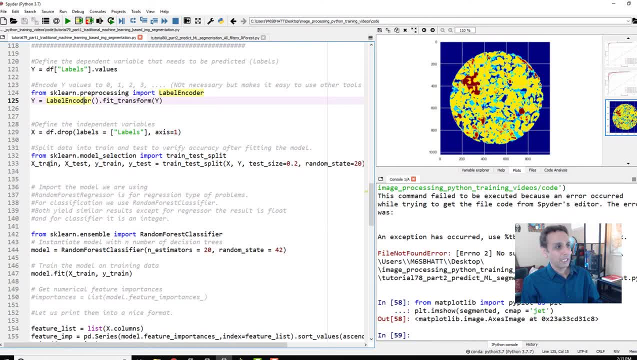 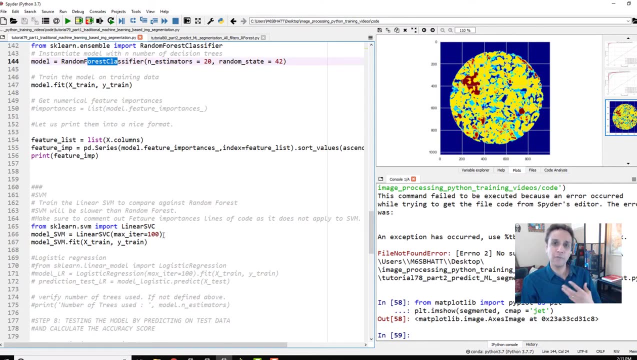 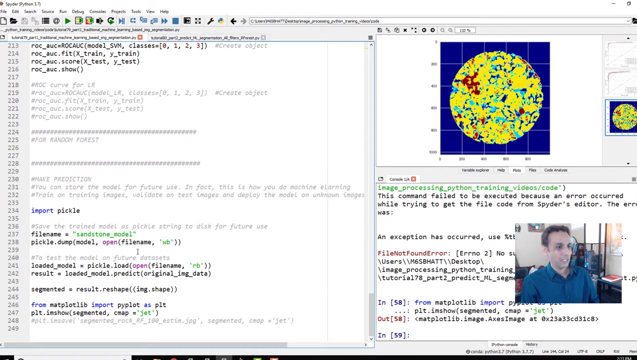 labels, which was an optional step. but eventually we divided our data frame into X and Y, where X is all the features and Y is the values, And we trained a random forest and we also trained support vector machines and we realized random forest gave us much better accuracy than support vector machines and eventually we saved the model. 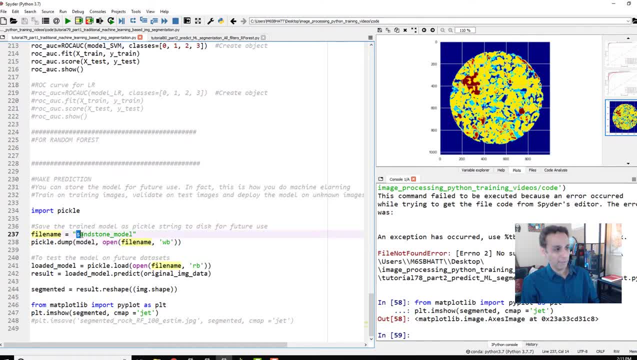 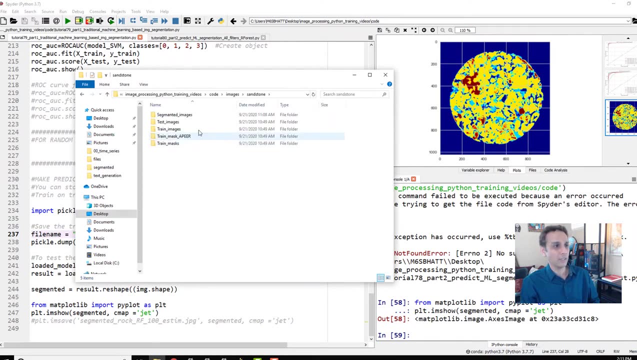 into a file name called sandstone underscore model. Okay, so so far, so good. now how do we take that model and segment? let's say we want to segment the model and segment the model and segment the model. let's actually look at the structure here. let's say I have a folder, let's go to segmented. 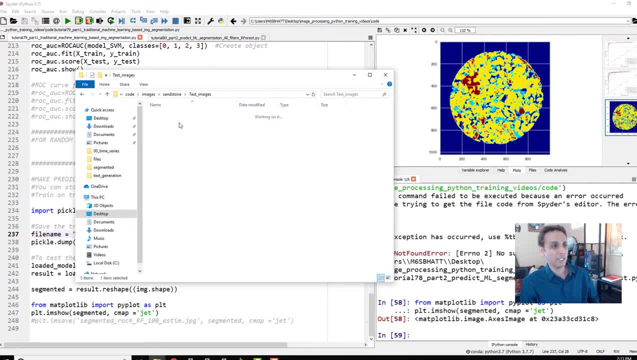 images. go ahead and delete everything we have there and test images. so I have about, let's say, five images, or in reality I have, for this data set, 1000 images that I would like to test, but of course I don't want to waste your time, so let's just pick five of these images at various depths. 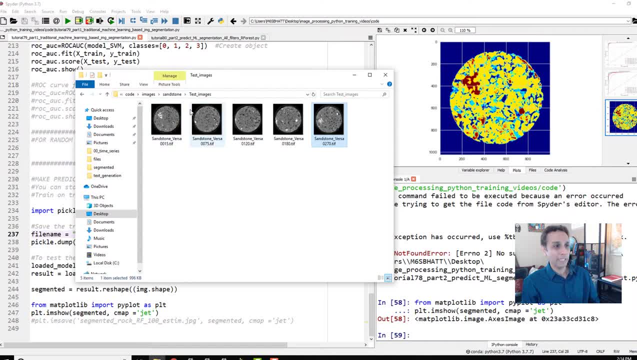 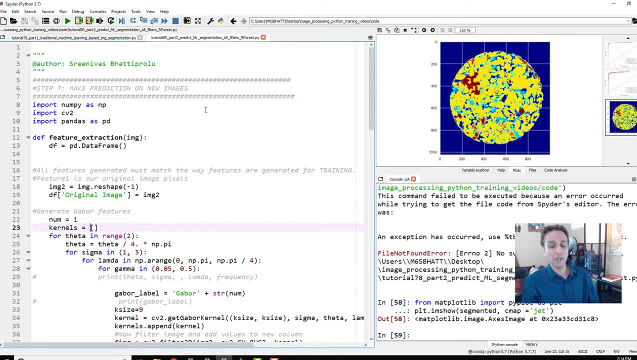 in this, in this image: stack and segment them, okay, using the model that we trained in the last tutorial. so how do we do that? so let's go to my part two: code again, all code will be shared via the github. look at the link underneath in the description. okay, so what do we do? there are many. 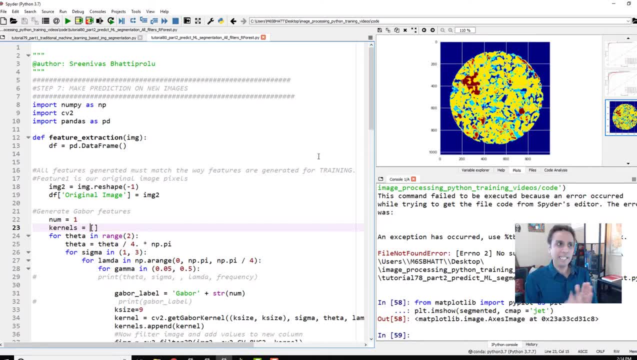 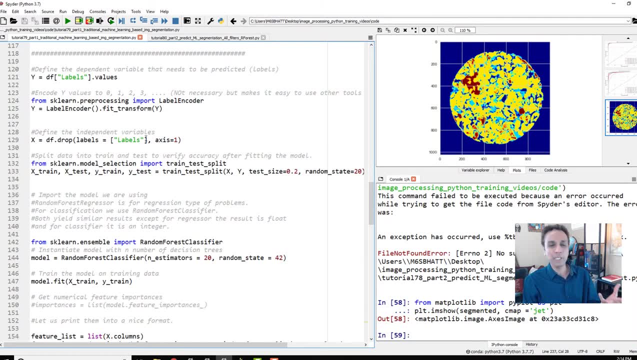 ways you can automate this process. but the whole point here is extract the features from each image exactly the way we did during training. otherwise it doesn't make sense. a Gabor one means should mean the same, okay. so first we have to read in an image, like we did before, right here we have to. 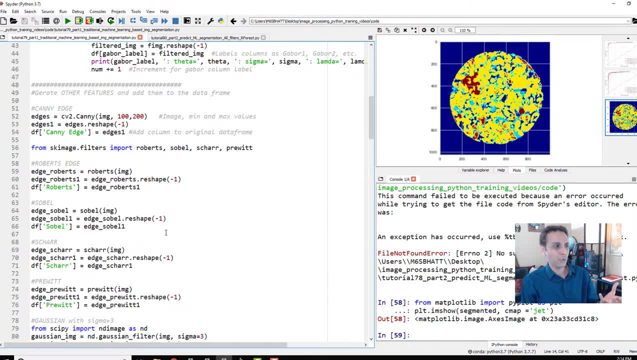 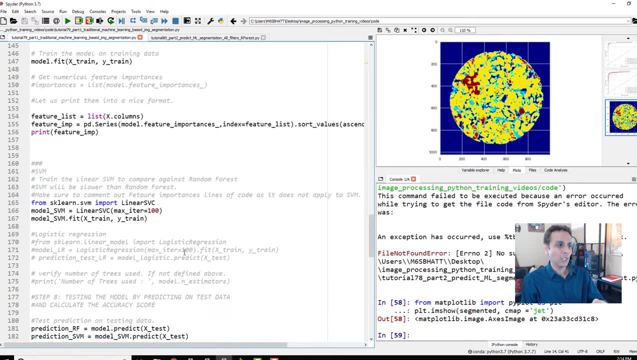 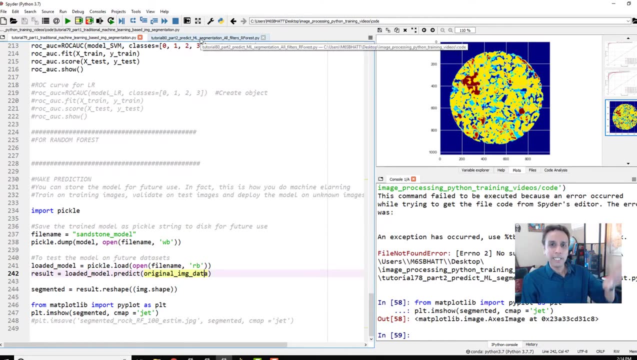 read in an image and we have to extract exactly the same gabor's, exactly the same other features and create a data frame and supply that to as an input to our trained model, just like we did here. okay, so I copied the entire code from here- most of it, okay, up to the training part- and I created 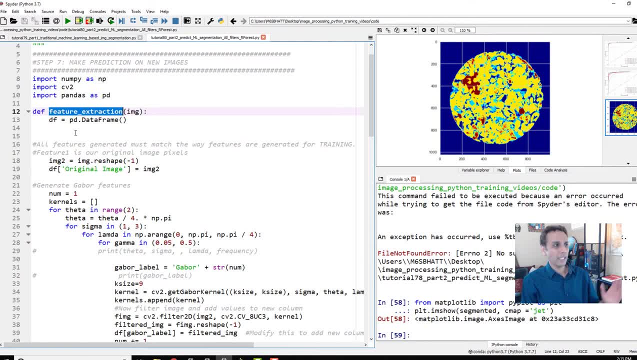 a function called feature extraction. okay, and I just tabbed everything. as you'll see, this is identical. so what I'm doing is I'm going to create a function called feature extraction. okay, and I just tabbed everything. as you'll see, this is identical. so what I'm doing is I'm going to create. 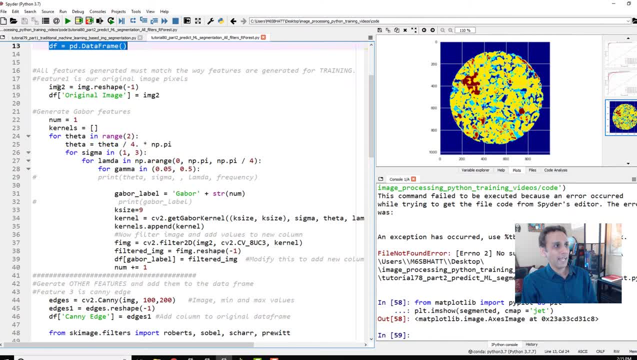 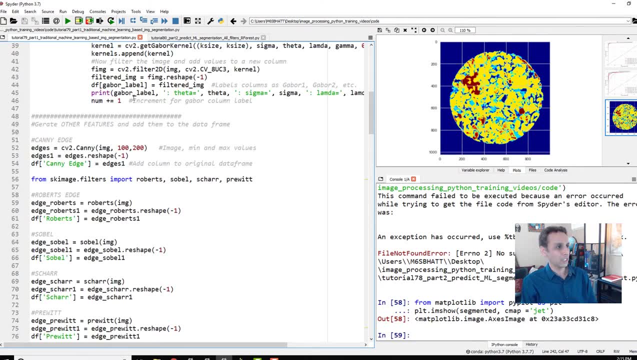 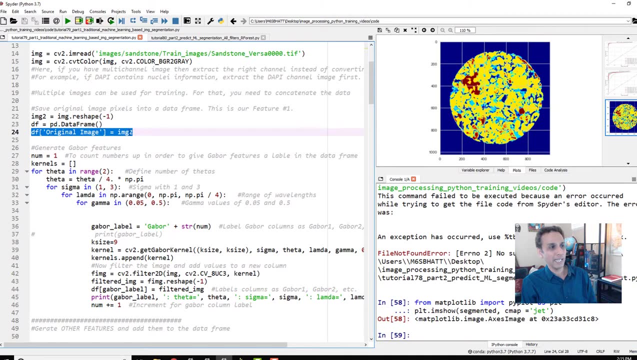 a data frame, empty data frame, and then to that add the pixels of original image. if I switch back to my previous tutorial, this is exactly what we have done initially. okay, we created an empty data frame and to that we added a column called original image and added all the pixels and 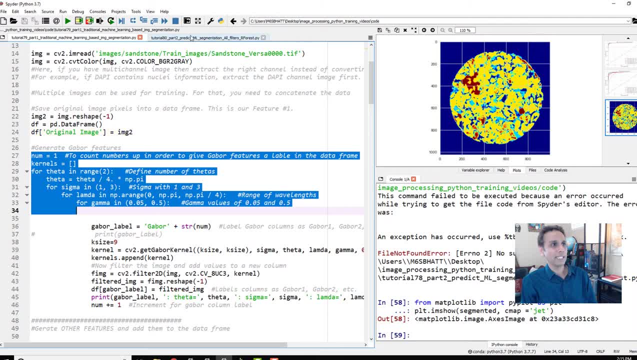 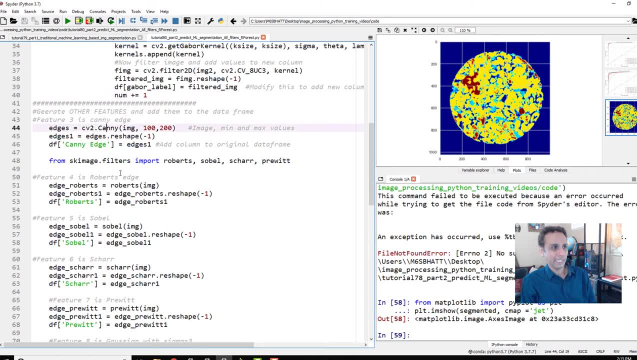 then we added Gabor to that data frame- exactly the same thing that you'll see here. so this is the first column, and then the other columns are added exactly the same way, and then canny and roberts and sobel- everything exactly the same. if you don't have the same number, 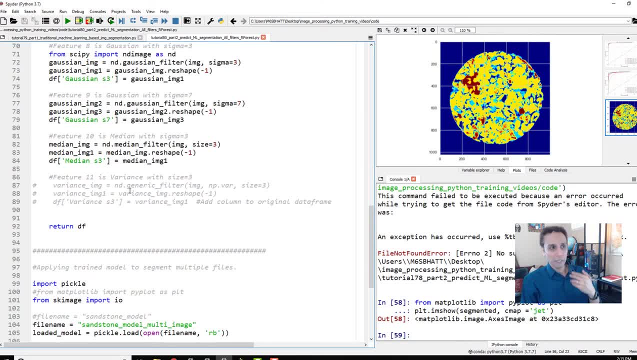 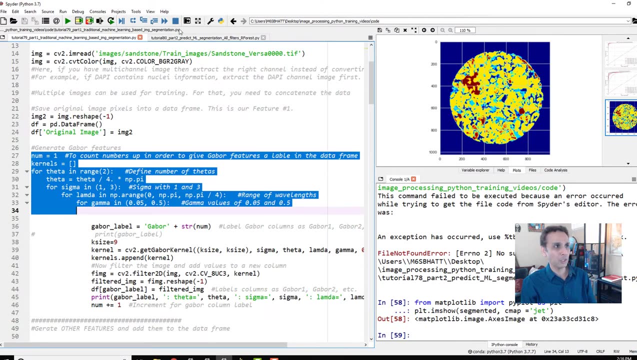 of columns, simna type of data, then of course it'll throw an error. even if it doesn't throw error, maybe sometimes you make mistakes that are not easy to catch, so you'll get wrong results and then you'll wonder why. so it's very important to go back and make sure. okay, both look very similar. 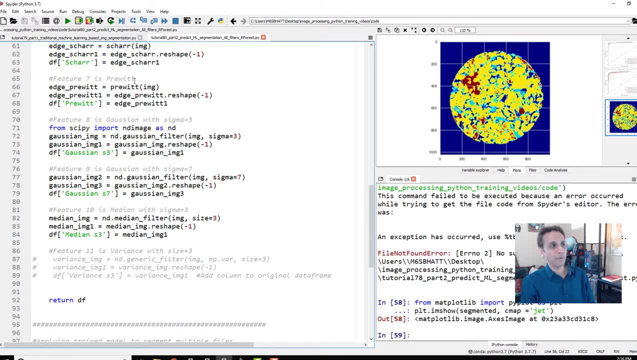 okay, in fact, the best thing to do is separate this feature extraction part and create a class by itself and then call that class into your training and also into your prediction. so any change you make, you know, in the feature extraction is applied, so you don't have to worry about this. so that's. I'll leave that for you, but for now we are capturing what 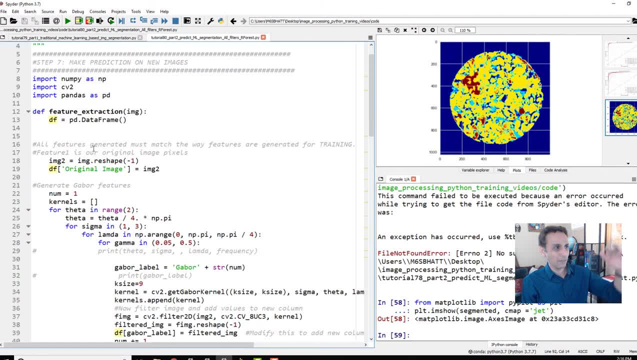 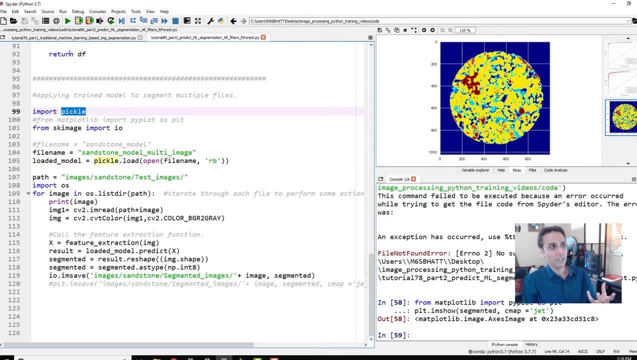 this function returns is a data frame. that's it, right? I mean all of this. it returns this data frame that contains all these values, and that data frame goes into our prediction. that's it. so how does it go? now? I'm importing pickle because our in the last tutorial we actually ended by 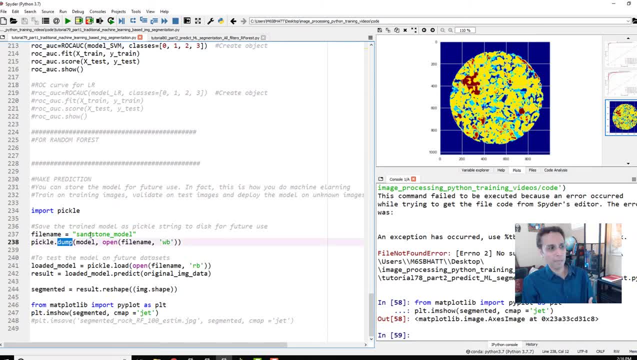 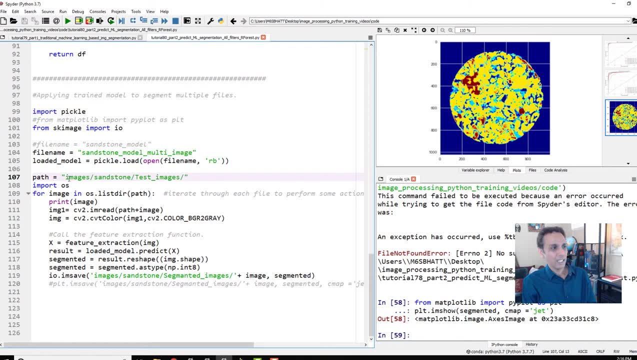 saving this, dumping this model as a pickled file. okay, so that's what we are importing here. so we are loading the model and then I'm giving a path of test images, sandstone slash test images- right, this folder path, and now I'm using oslistdir or you can use glob. it's a. 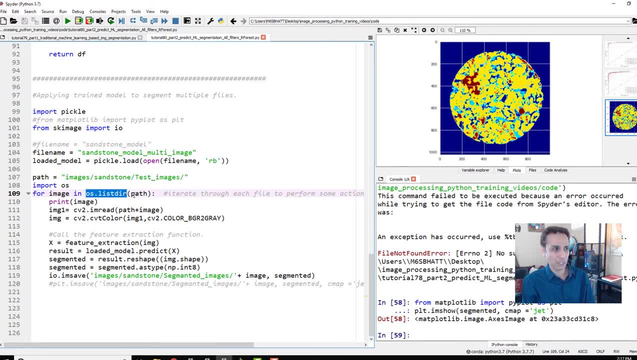 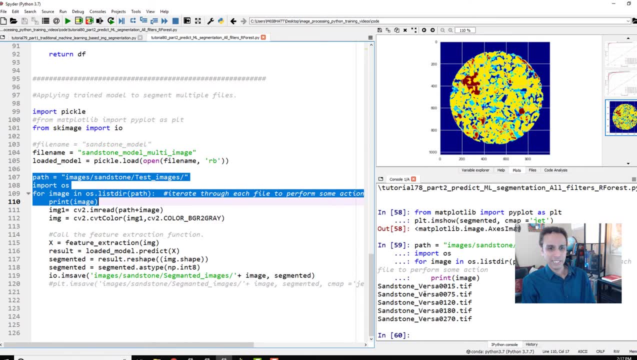 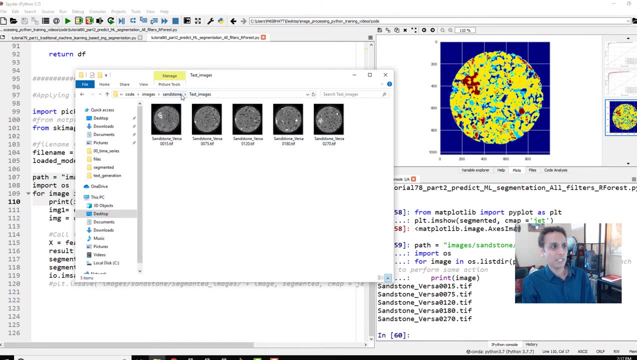 zip file. if that's what's up to you, to walk through the folder, through each image, okay. so, in fact, if I just do these lines for now, you should see that it's reading these file names: 15, 75, 120, 180 and 270, right? so these file names, and once we have the file names, I'm just doing. 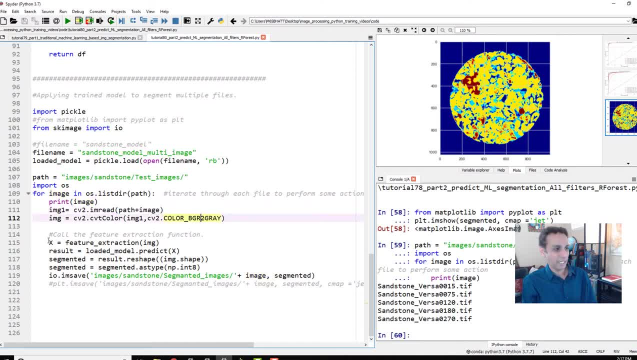 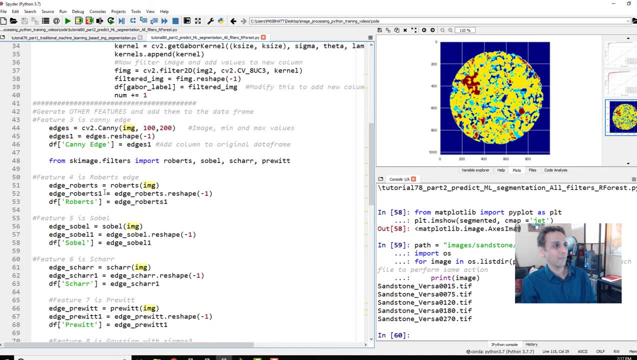 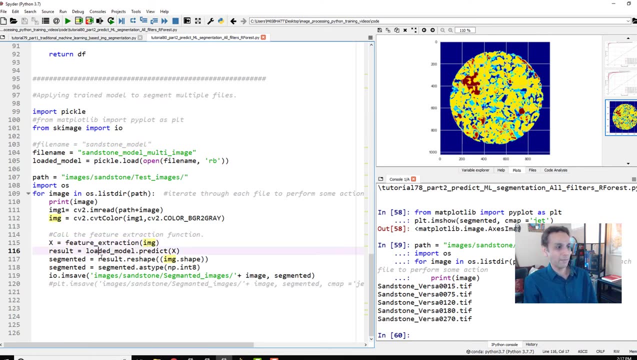 im read, just like the last time, converting that into gray and then extracting the features, which is feature extraction, on my input image. what does it do? feature extraction? it just runs this function. yeah, so let's go ahead and do that. and then, uh, that is my result, and my result is going to be one single column. i need to reshape. 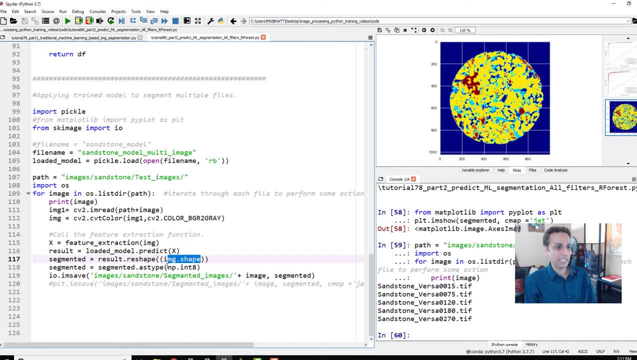 it into my original image shape and i'm converting that into integer 8. otherwise that would be integer 64 and when you save it sometimes it may give some throw some weird errors depending on the version of python you're working on. but i am converting each of these- uh, you know, into 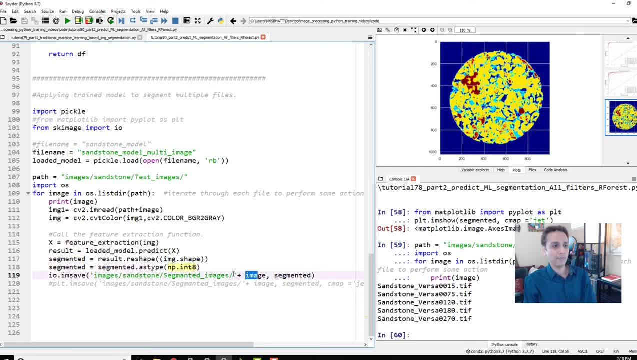 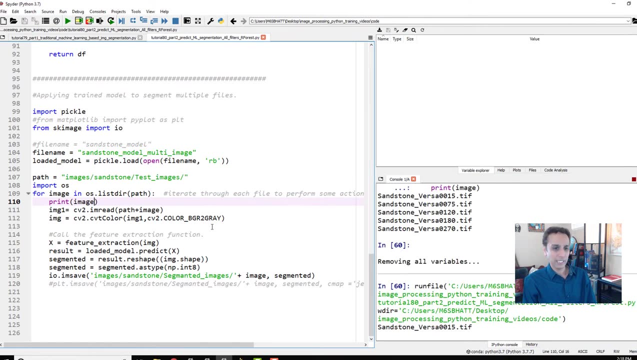 integer 8 and then saving it into a different folder called segmented images, with the same file name as my original image name. please read this: and now let's remove all variables from our previous run and just run this and the first step. sandstone versus 0: 0, 1- 5. 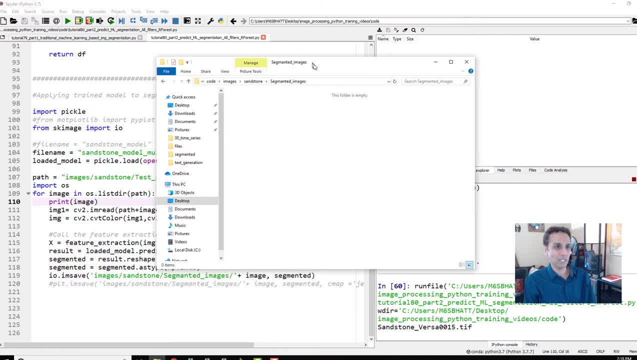 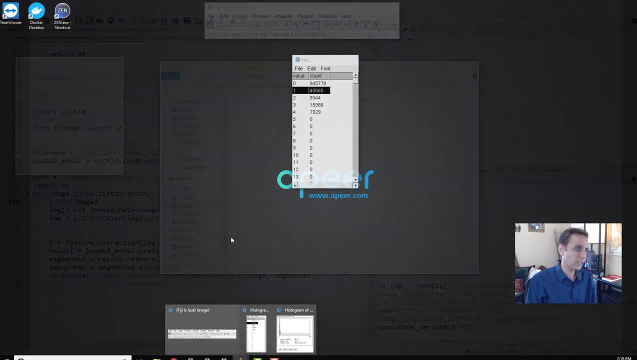 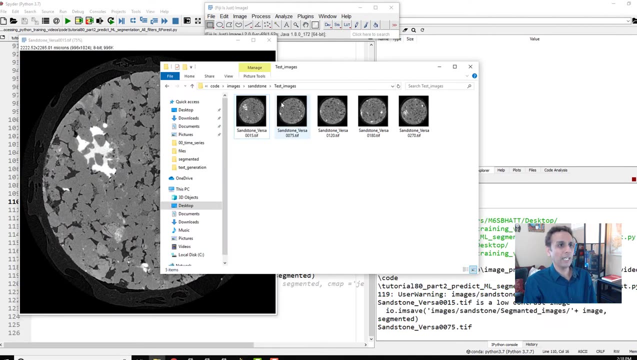 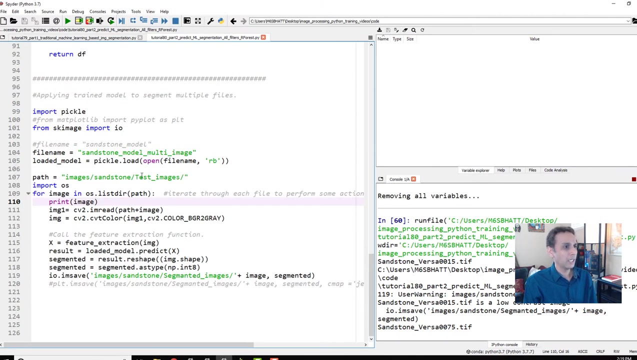 and if i open segmented images, i should see a result any moment now. so let's, in the meantime, open our input images. so, in fact, let's go back test image and open the first test image and then look at the result. we are back here and oh, i did a mistake here, so let's go ahead. and i mean it did save it. 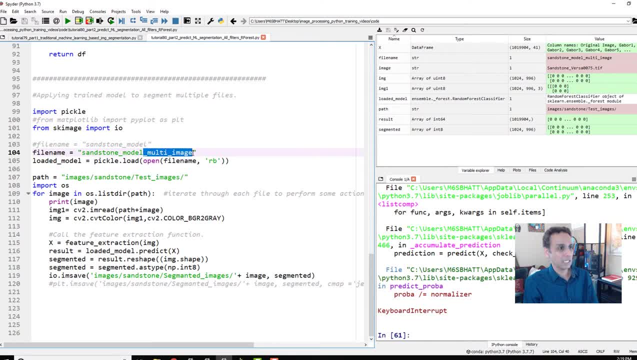 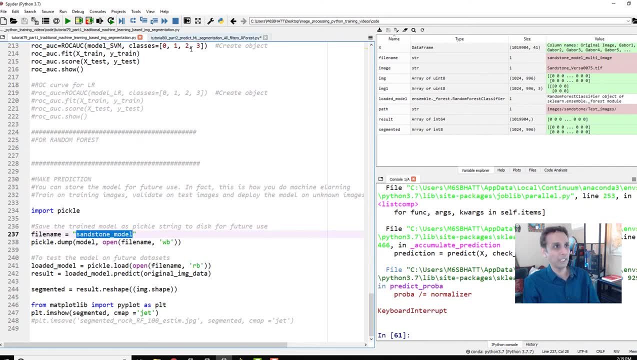 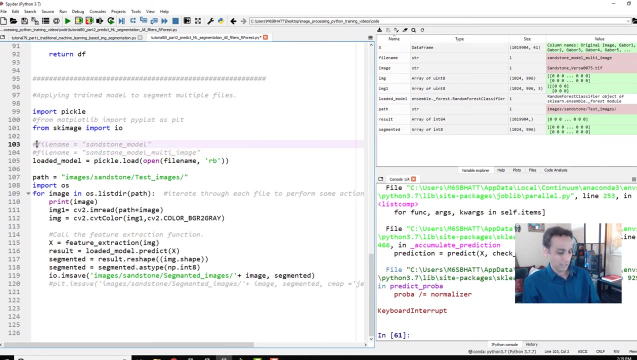 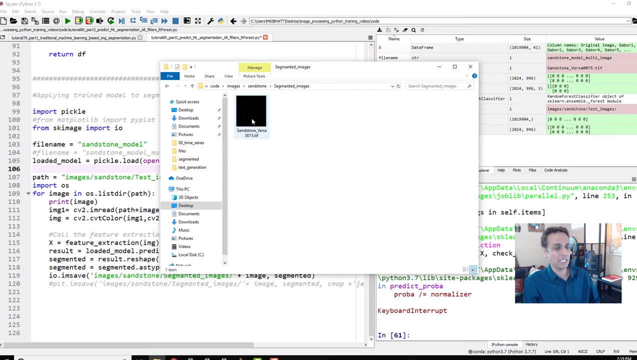 i should read something called sandstone underscore model, the one that we just saved, sandstone underscore model, not the other one. so sorry about that. let's do this one more time. in fact, let's, let's do that, okay. so let's run this. let's clean up our segmented images. 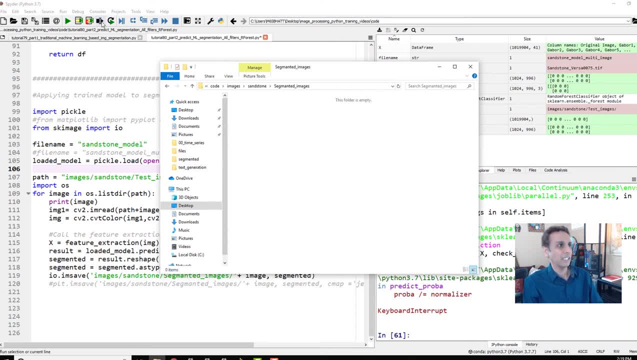 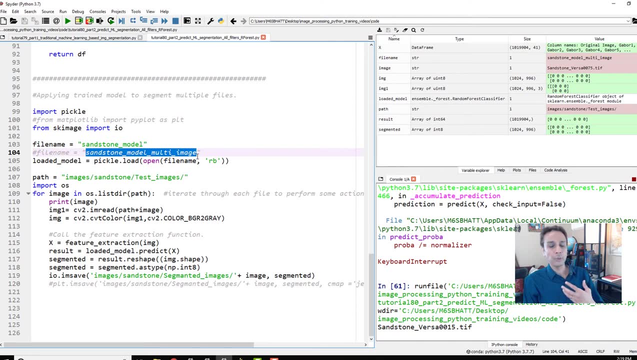 remove the one that it segmented already and then run this one more time. okay, so the other sandstone model, multi-image- is the one we are going to do in our next tutorial, where we're going to use multiple images for training, which means the result, hopefully, would be more. 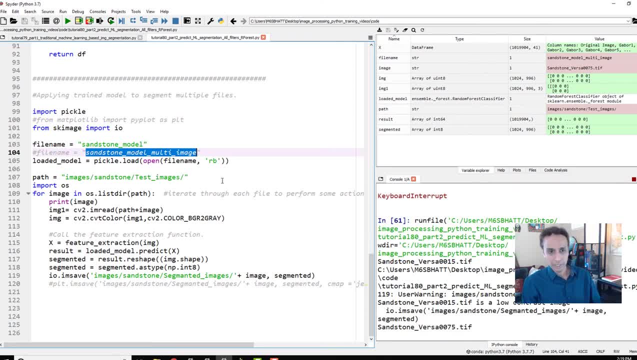 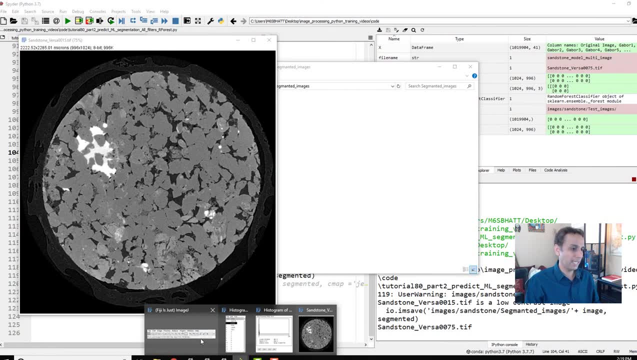 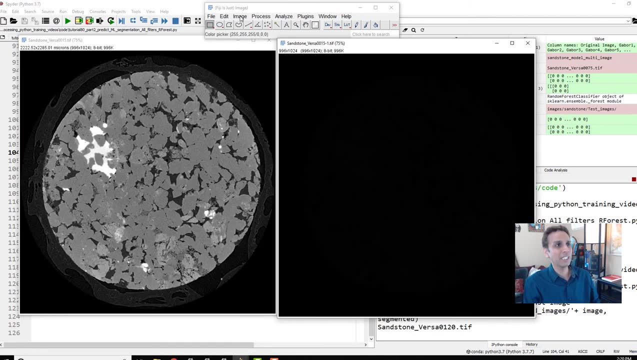 accurate compared to what we are getting right now. so image number one is done already, so let's go ahead and have a quick look at that image. so this is the raw image and how does the segmentation look like? and there you go. that's our segmentation. you don't see much of anything. that's because 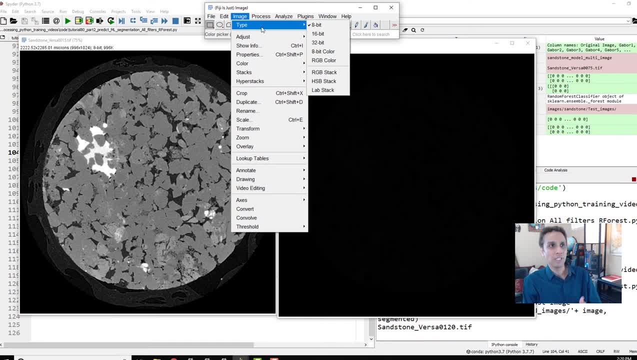 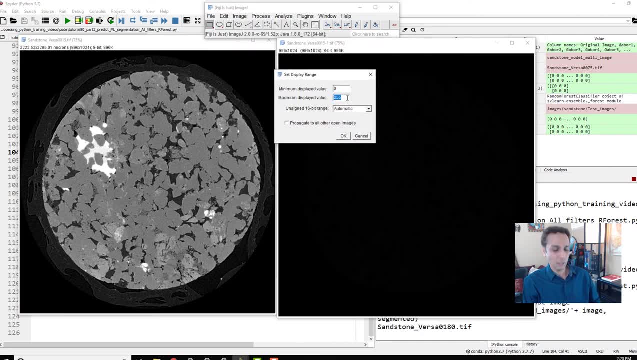 of the image. so let's go ahead and run this one more time. our pixel values are, if you remember, one, two, three, four, so let's go ahead. and or zero, one, two, three. sorry, we encoded this in this case, so let's go from zero to three, and there you go. so this is. 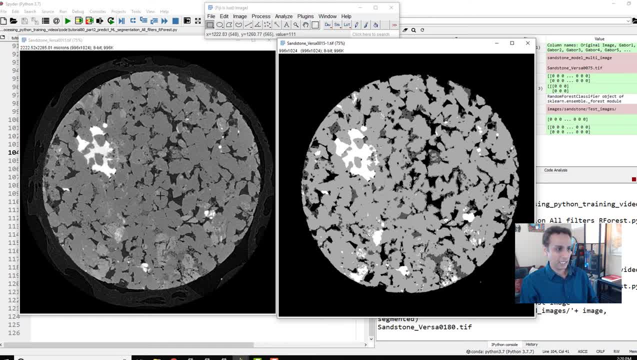 our result and this is the actual image, and that is not bad actually, and you see, down here it's showing up as bright pixels. it is brighter, but not that much brighter. so hopefully we'll get better results when we have more labeled data. you can label more pixels in one single image. 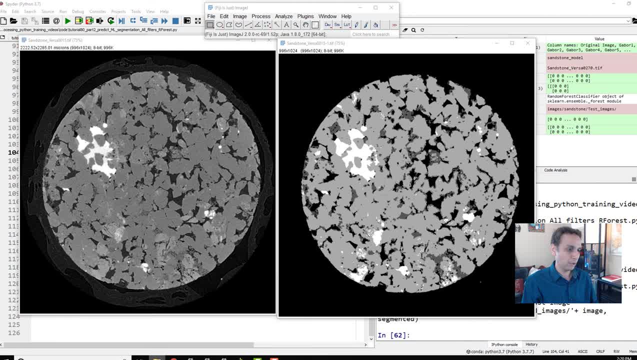 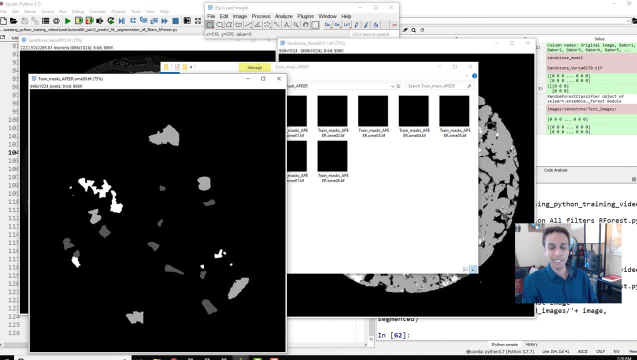 what do i mean by that? i think you know what i'm meaning, uh, but let's go ahead and check that. the mask that we used for this is, uh, it looks like this: not many pixels. you can actually, uh, be very patient and label a whole bunch of these in here.